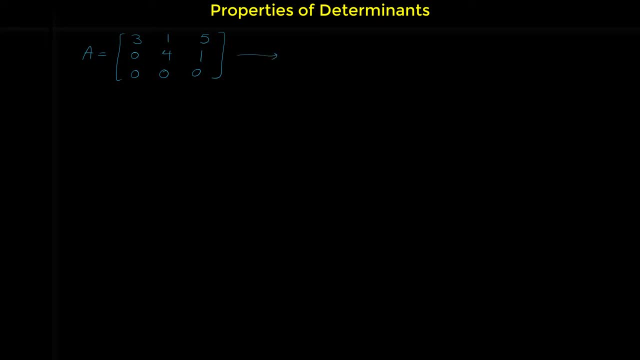 of that row is zero. so, without finding determinant of this matrix, we know that determinant of this matrix is zero. Let me show you another example, 2 by 2 example. Consider this matrix: 0, 5, 0, negative, 3. Note that this notation, when we use vertical lines, this means that we are finding determinant. 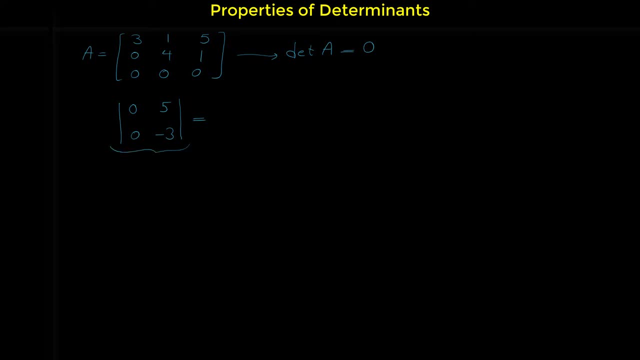 of the matrix, not the matrix. so this is the symbol for determinant of the matrix. and determinant of this matrix is zero because this column, all the elements of this column, are zero. so determinant of this matrix, without calculation, is definitely zero. This is the first property. The second property that we want to talk here is that if in a matrix two rows or two columns, 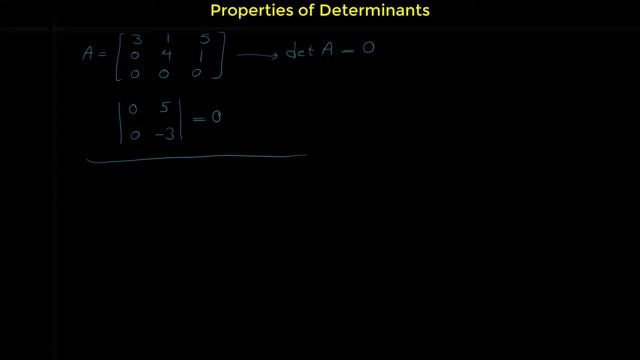 be a factor of each other, then determinant of that matrix is zero. Let me show you this by an example. Consider this matrix: 1 negative one. three zero four. seven negative two, two negative six. Pay attention: in this matrix, this row is a factor of this row. actually, if you multiply. 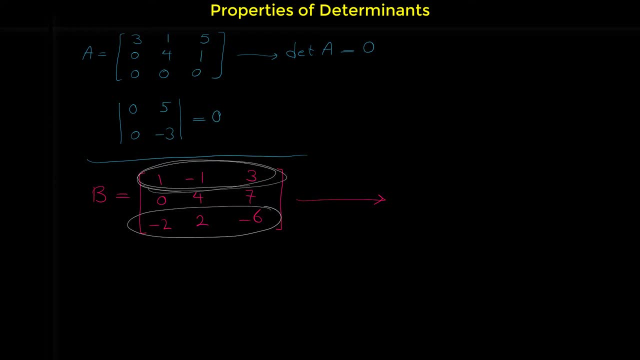 this row, the first row, by negative two you can get to this row. so if you multiply every element in this row- negative 2, 1 times negative, 2 is negative, 2, negative 1 times negative, 2 is positive 2 and 3 times y negative 2 is negative 6.. so, without doing any calculation, 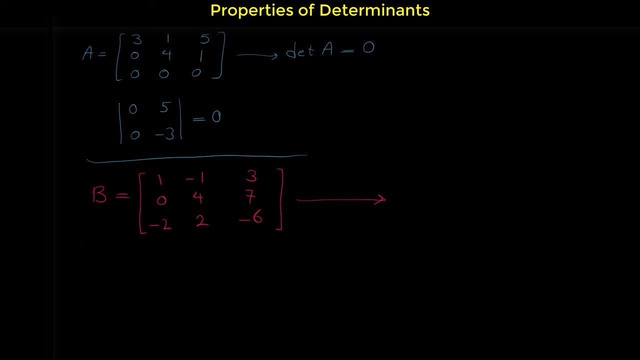 from this property. we know that the determinant of the matrix b determinant of the matrix b is zero. so the reason that this determinant is zero, big is because this row is a factor of this row. let me show you another example. look at this matrix. let's name it c. 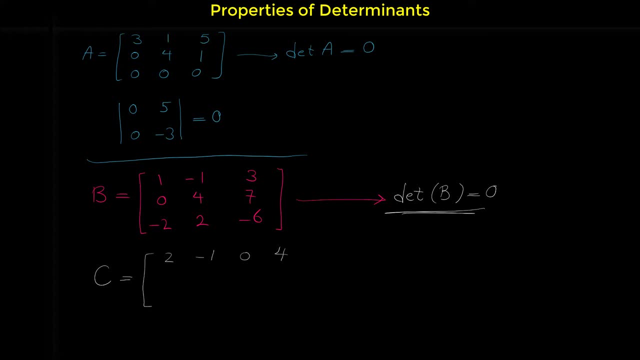 2 negative: 1, 0, 4, 1, 4, 3. 2 negative 1, 5, 7. negative: 2, 3, 0, 0, 6. if your attention in this matrix, because this column is a factor of this column, if you multiply this column by 2, you can get to the next column. two times two is four one. 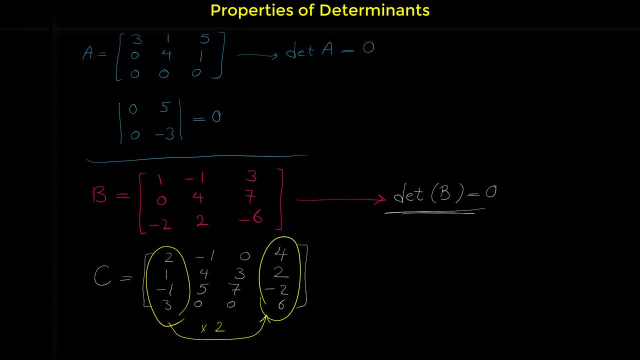 times two is two negative. one times three negative two and three times two is six. so this fourth column is a factor of first column. so determinant of this four by four matrix is zero. now let's talk about the next property. if you switch two rows or two columns of a matrix, 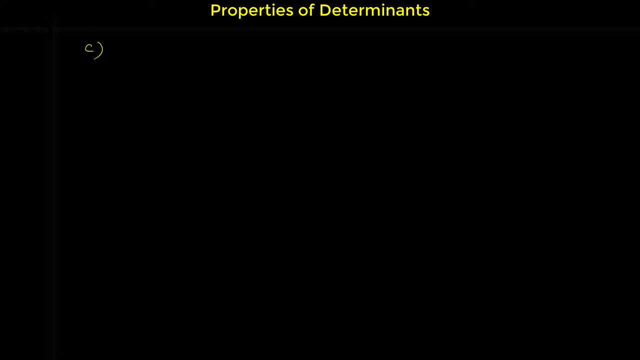 the terminal of the matrix becomes negative of the original value. let me show you this by an example. let's suppose we have this matrix, matrix m, let's name it negative one, three, five, seven. determinant of this matrix is negative one times seven, which is negative seven minus three times five minus 50. 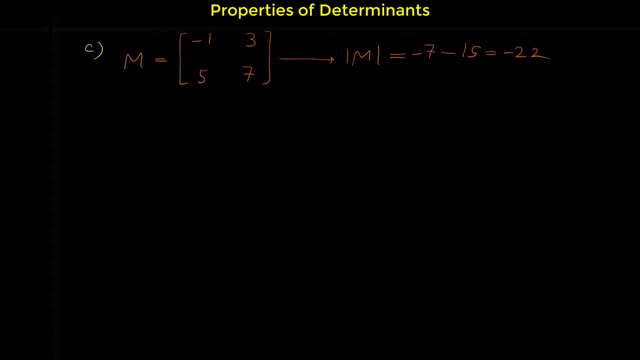 and this equals negative twenty two. now let's switch two rows of two columns. matrix n: let's switch this column with this column. then we have this: matrix 3: 7. negative 1: 5 because we switch two columns. the determinant of this matrix, without any calculation, is negative. of this value, it should be positive 22. 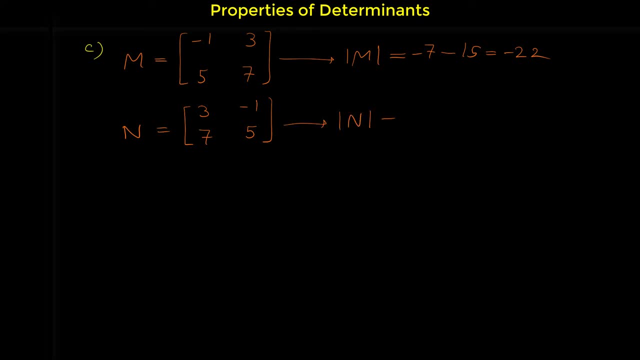 let's see what is the terminal of M: 3 times 5 is 15 minus negative seven. minus these times this, 15 minus negative 7 is 22. this is an example that shows that if we switch two rows or two columns of a matrix, determinant of the matrix. 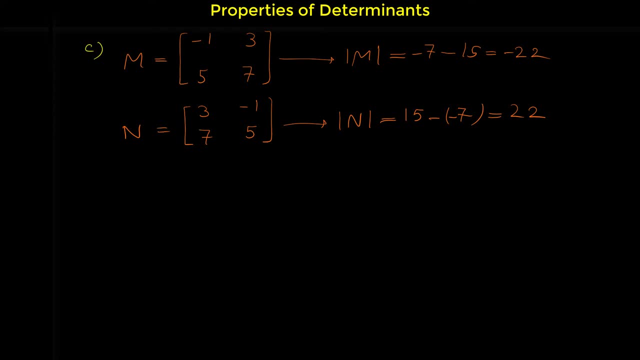 becomes negative. note that here we are not proving these properties, just we are reviewing these properties and sometimes these properties. this can help you to find the terminal of the matrix easier. if in a matrix we multiply a row or a column by constant, by any number, the terminal of the matrix multiplies by that number. 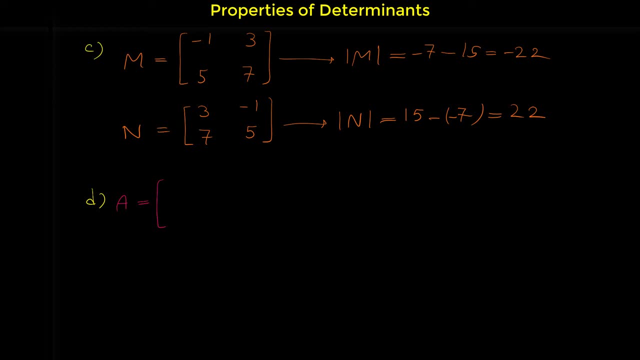 let's say we have matrix a with these elements one, three, two, five. so the terminal of this matrix is one times five minus three times two is negative one. now if we multiply, let's say, the second row by 10, for example. so we multiply this row by 10.. let's see what happens to the 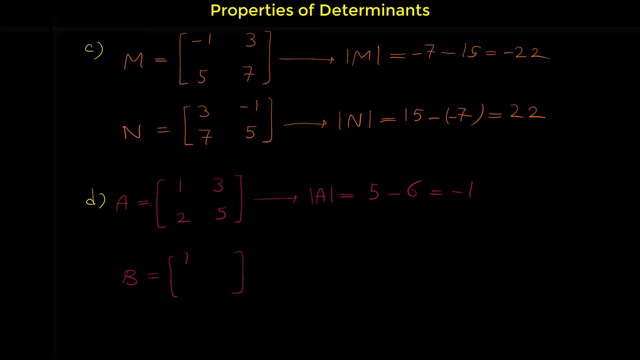 value of the determinant. if we multiply the second row by 10, then we have 20- 50.. because we multiply this row by 10, the terminal of the matrix b should be negative 1 times. so again, when we multiply a row or a column by number, 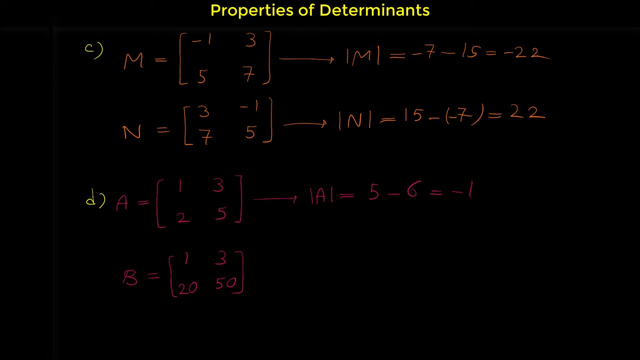 the terminal of the new matrix is determinant of the original matrix multiplied by that number. let's see is it true or not? the terminal of the matrix b, if we want to calculate, is 1 times 50, which is 50 minus 3 times 20 is 60 and 50 minus 60 is negative 10.. this example confirms our property. again, i should. 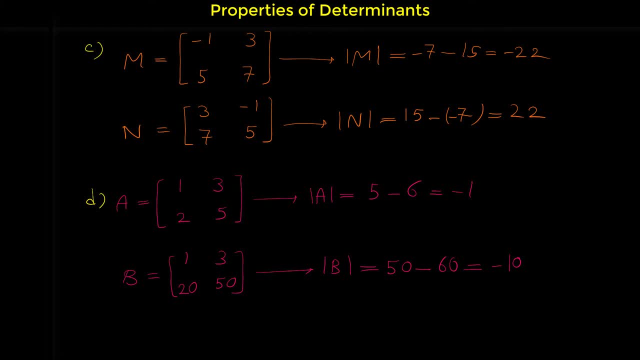 mention here. we are not proving these profits, just we show an example of those properties. let me show you another property. if we add or subtract a factor of one row to another row, or if we add or subtract a factor of a column to another column, the terminal of the matrix doesn't change. let me show you some examples of this property. say: 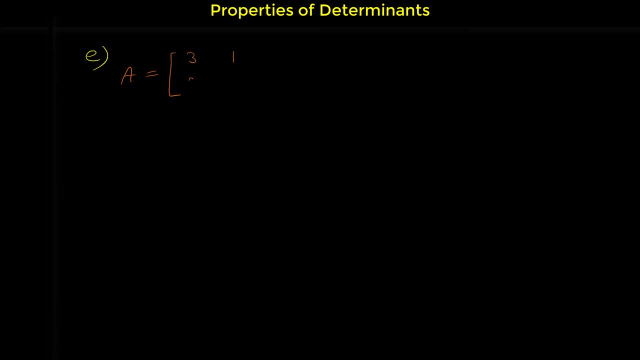 we have this matrix: 3, 1, 2, 6. the terminal of this matrix 3 times 6 is 18 minus 1 times 2 minus 2 equals 60. now let's multiply this row by number and add that to the next row. 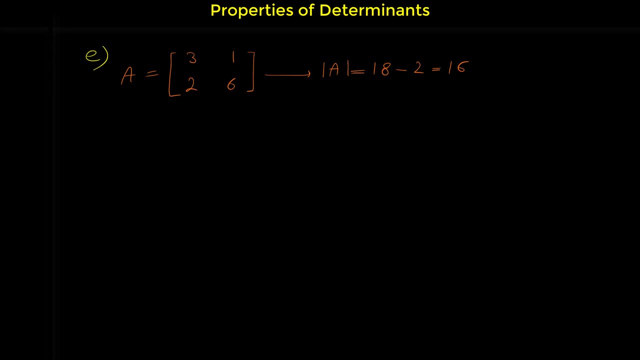 so we want to multiply this row by a number and then we add that row to this row. let's, for example, multiply this row by 5. if you multiply this row by 5, then we 3 times 5 is 15. 1 times 5 is 5. if we add this row to the second, to the, 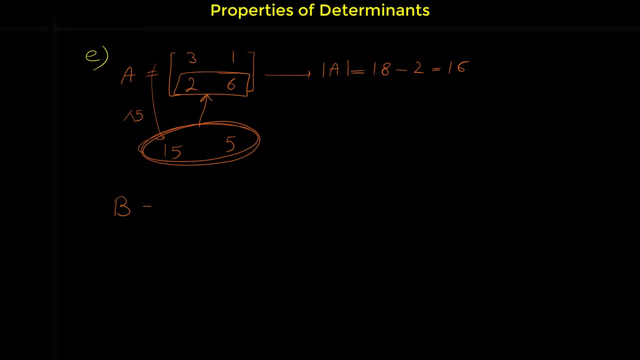 elements of the second row. we get to this new matrix, so we are not touching the first row, we are leaving them 3: 1. but we are multiplying this row by 5 and then we add that to the second row. so if we add this to the second row, 15 plus 2 is 17, 5 plus 6. 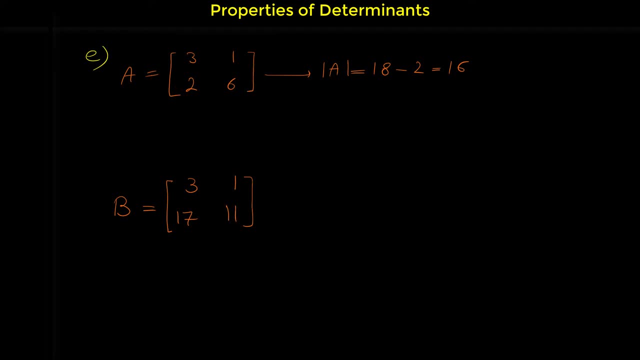 is 11.. now we can see that the terminal of this matrix is the same as the original matrix. it's really interesting. let's see, really, the terminal of the matrix b is still 16 or not. 3 times 11 is 33. 17 times 1 is 17. 33 minus 17 is 16.. as you can see, the terminal 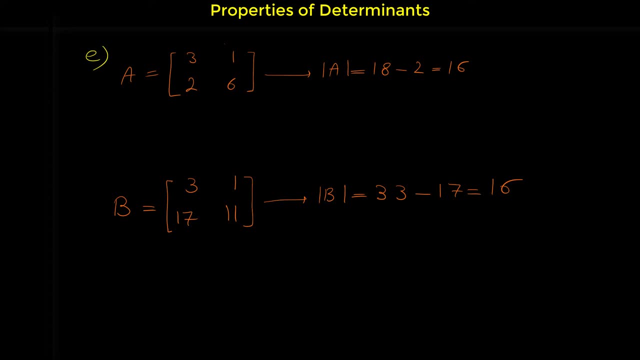 is the same. note that it doesn't matter the matrix to be 2 by 2, 3 by 3, 4 by 4, 10 by 10. for any matrix, if you add a factor of one row to the other rows, the terminal doesn't change. if you add: 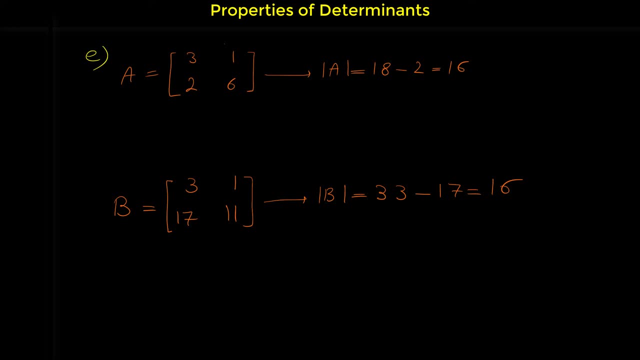 a factor of any column to the other column, the terminal doesn't change. let me show you another example in this case. say we have a matrix like one, two, three, four. the terminal of the matrix m is one times four is four minus two times three is six. four minus six is negative two. now, for example, let's add a factor.